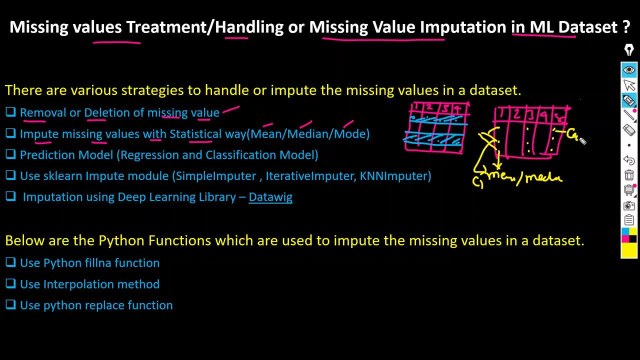 this missing value. Let, this is your categorical column. So we use mode of this column and, whatever the value we get, we impute this missing value with the help of this value. And after that we have discussed prediction model. In this prediction model, what we used, 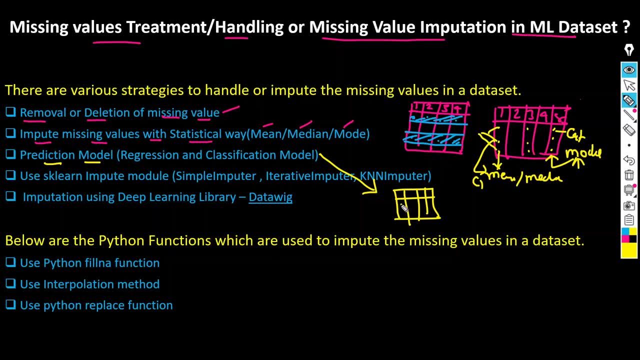 to perform. let, this is your data set And there are some missing value in this data set. So first, we predicted these missing value with the help of prediction model. Once we have the predicted output, these output is corresponding to your missing value, So we impute this missing value using these output. 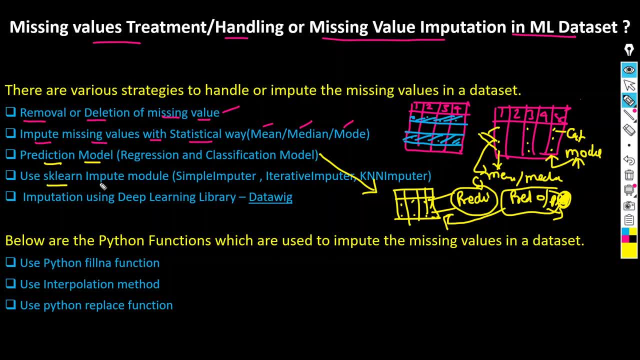 Now, today we are going to discuss about the ascare- learn impute module, Ascare- learn impute module, which has three class: simple imputer, iterative imputer and knn imputer. So first we are going to discuss about this, then we will discuss iterative, then we will discuss. 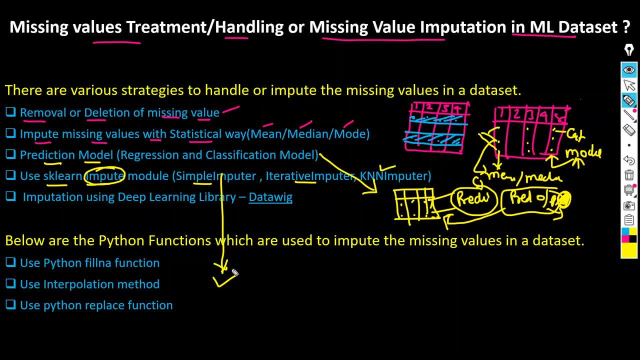 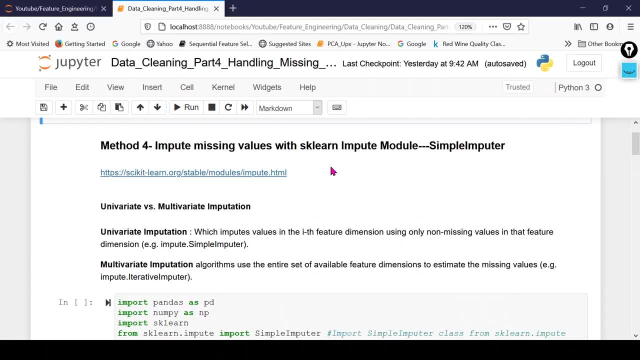 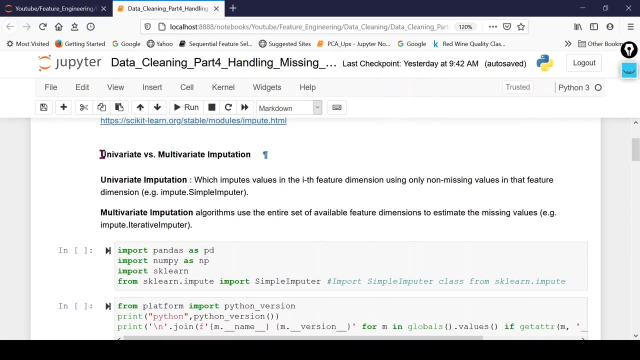 knn imputer. So let's start. Let's start our Jupyter notebook and try to use simple imputer- how it performs- to impute the missing value. Here you can see that we normally have univariate and multivariate imputation in the real-world data set. Univariate means once we impute the missing value, one. 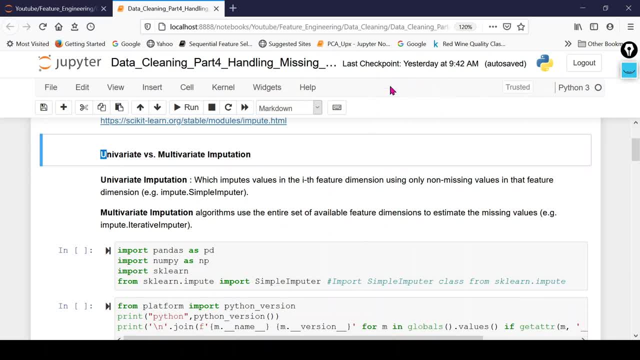 by one. It means we take first column and impute that column, And multivariate means 2 or more than 2. We take 2 columns and impute all the missing value on these two columns. So univariate imputation be perform by using the simple imputer. And if we want to include 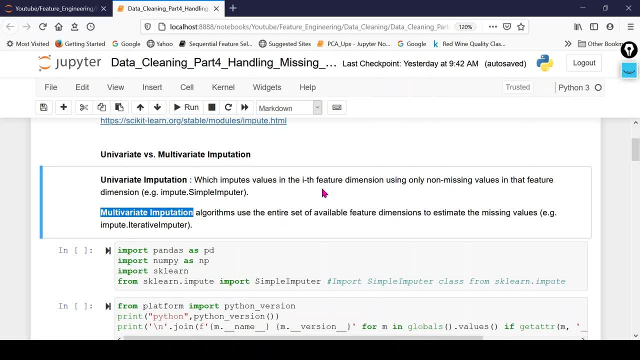 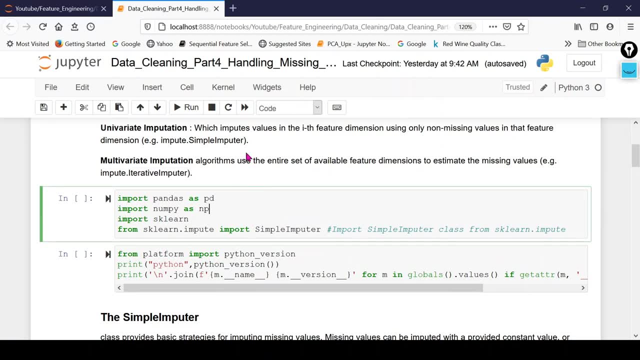 the multivariate imputation. it means two or more than two variables. then we use iterative imputation. So let's start. So here I am going to import the some libraries which I Am going to use to perform the dirty state work in the maintained mano-file of progress variable arriving in a 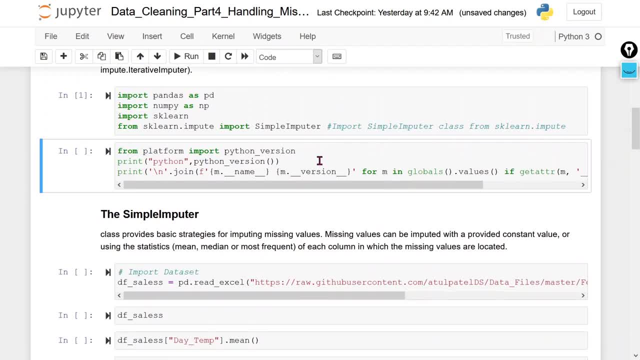 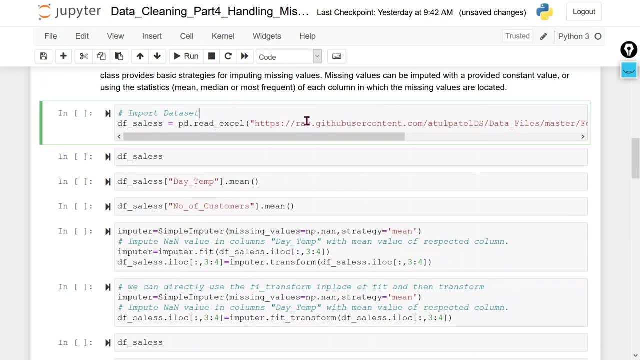 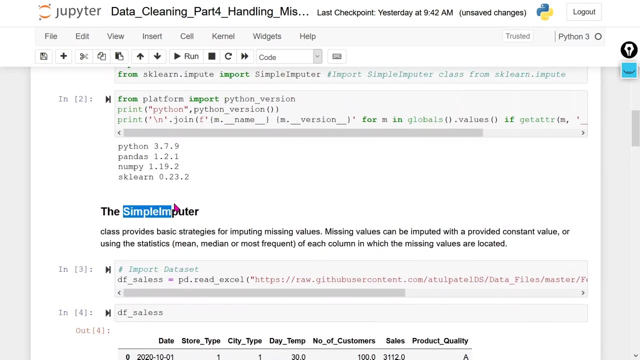 the simple imputer. so here I am going to print the version of the imported libraries. this I will explain you in couple of seconds. here I am going to import our data set, which I created manually. now let me describe this simple imputer. how does it work? by using this data set. first, let me 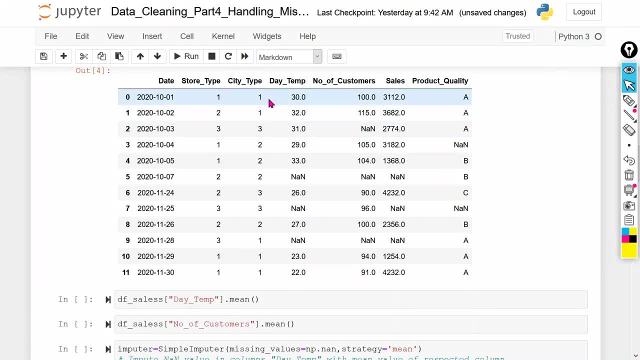 explain theoretically how does it work. let's, we want to impute this column and this column, and this column and this column. so this is your numerical column, this is your numerical column. this also is numerical column and this is your categorical column. so, by using the simple imputer, 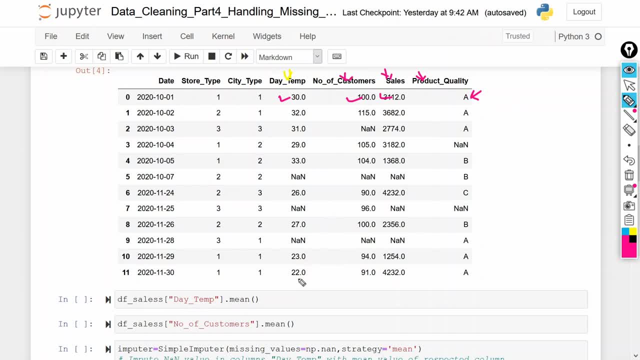 we impute the missing value one by one. first we impute, we take the column one and impute, and then we impute in other column, then we impute in other column. so it means in a single go we can take all these three column and we can impute the missing value. but point to be, 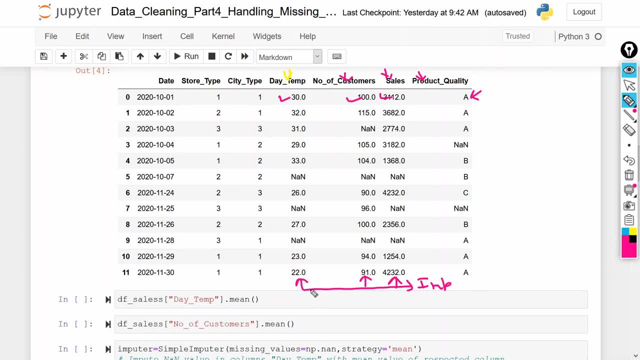 noted here. we cannot impute this column with the help of C2. it means all the column imputation will be happen individually. so it means how we will impute. there are some strategy we use. we use some strategy for numerical column. 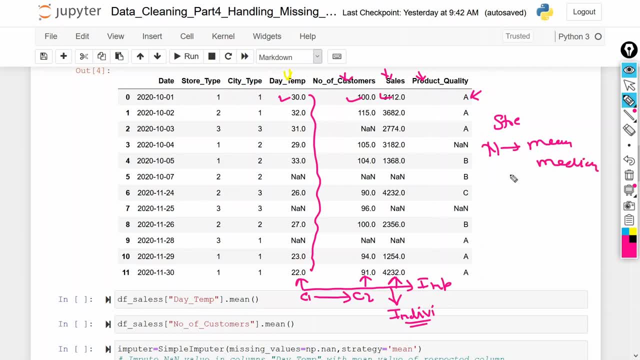 we use mean and median. for categorical column we use most frequent and constant. so if we want to impute this column, so what we will do, we will use simple imputer and we will use strategy mean. it means whatever the mean of this column, that mean value will. 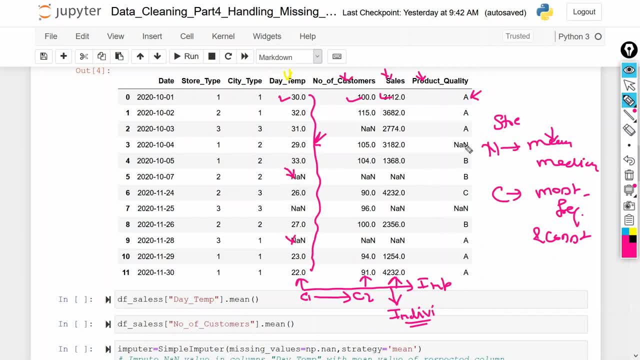 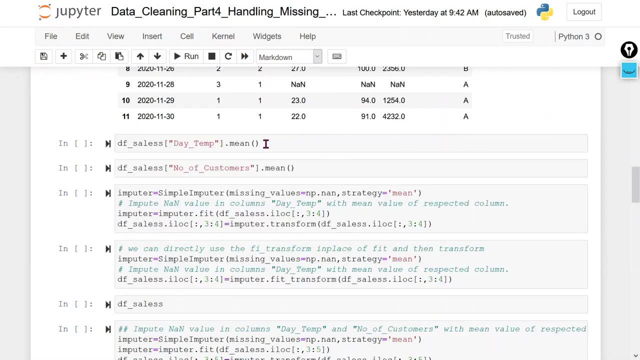 be imputed here, and same for categorical column. whatever the most frequent value we have in the column, that value will be imputed here. or if we want to impute any constant value or static value, then we can use the constant strategy. let's do by some hands-on. now i am going to take mean. 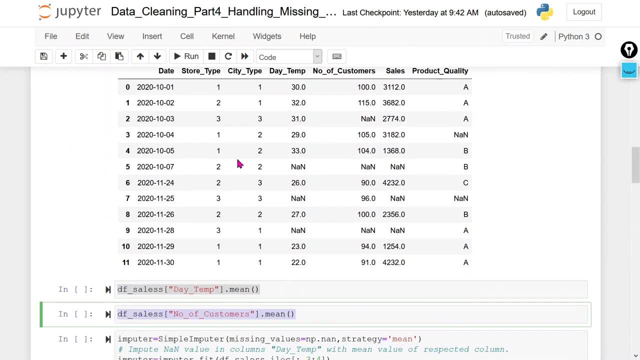 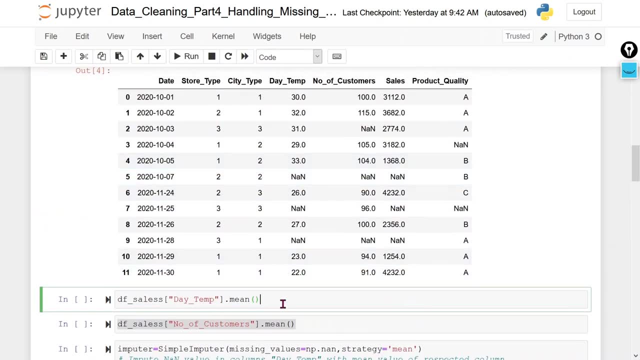 of these two column. why i am going to do? because we want to use this value to verify whether our simple imputer is working fine or not. it is just for the verification. so these are the mean value or the average value, so let's verify by 1.. are they also in this column? so let's verify by 1.. 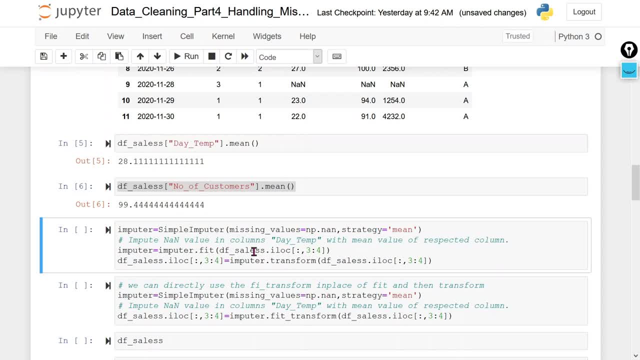 verify whether these are the value will be imputed by this simple imputer or not. So what I am going to use, I am going to first install our simple imputer, And strategy is mean. Now I am going to fit our which column? 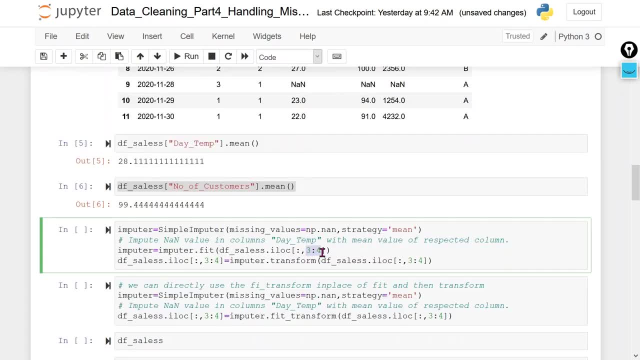 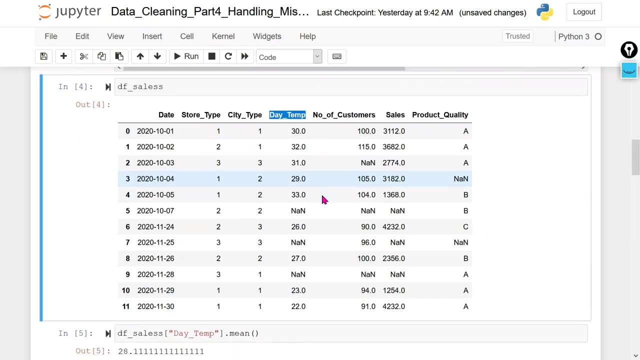 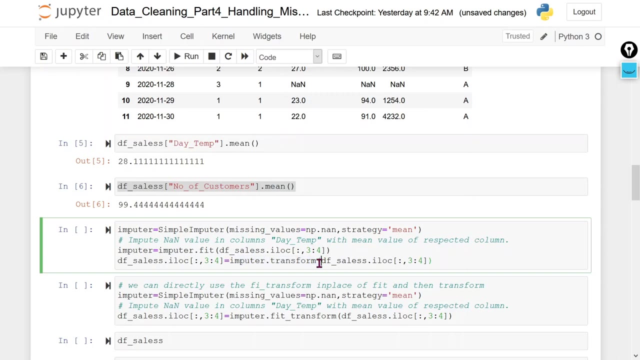 I am going to fit our column day time: 3 to 4, 0, 1, 2, 3 to 4 means 3 will be only count, So we will impute date, time. And after that what I am going to do: I am going to transform. after imputation, we transform. 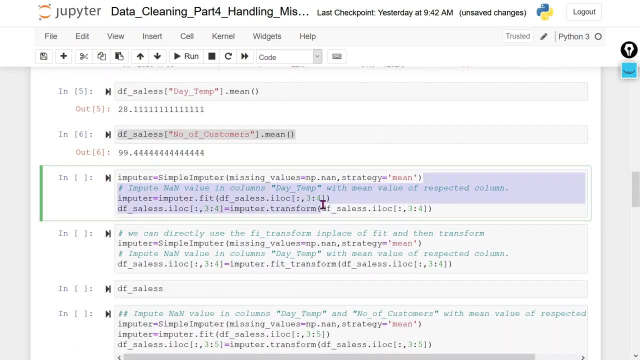 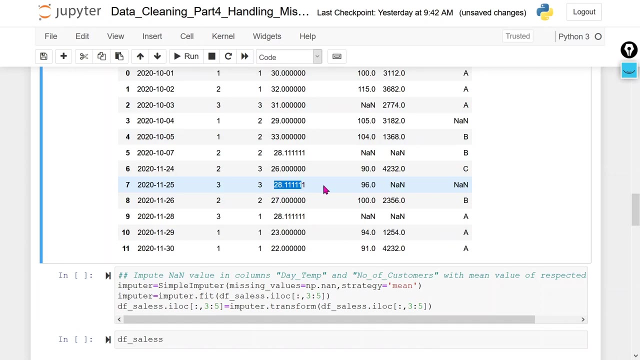 which data This particular column Till here, what it will do. it will calculate the mean and after that that mean value will be transformed over this column. So let me display here you can see that 28.11 has been imputed here. 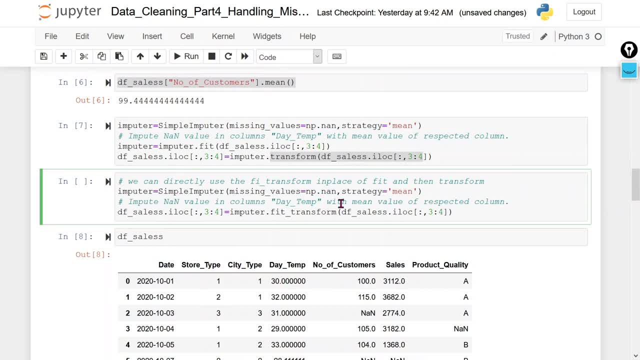 Same value. we are getting here Now in the second column, what I am going to use. I am going to use the. if you see here, first be fit, then transform. We have another method that can do in a single go: Fit and transform both in a single go. 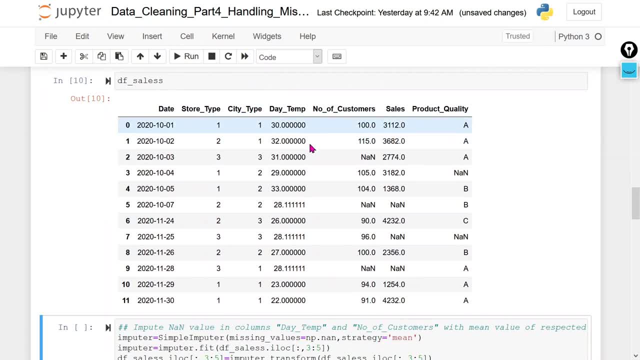 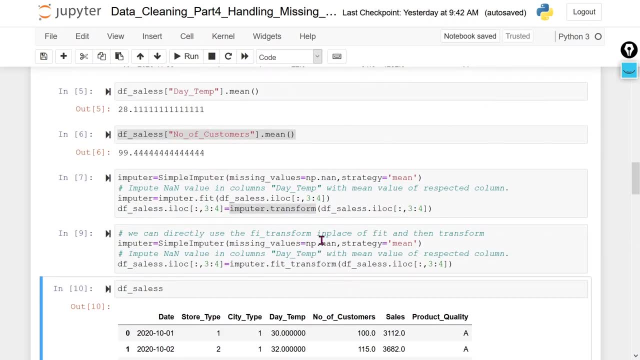 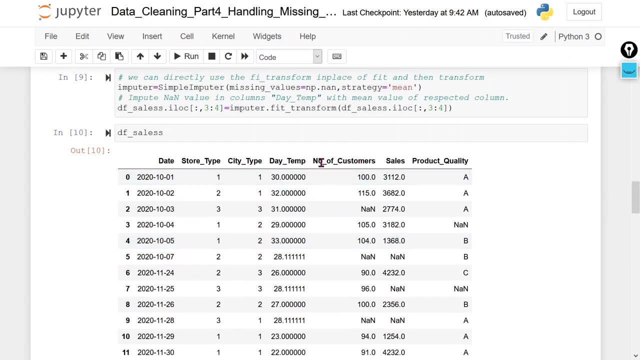 Let me do it. then again run it. It will impute same mean value here. It means I am going to use either method. Now, what I am going to use: I am going to use two column imputation in a single go. 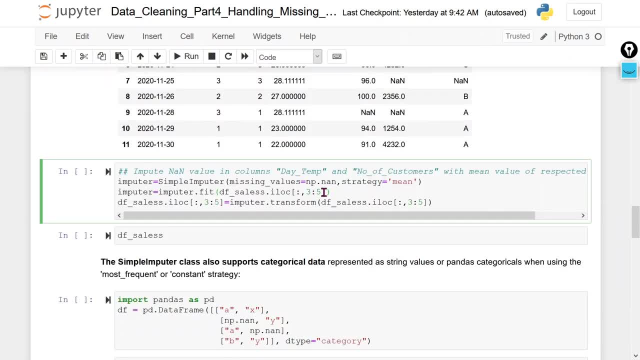 But both column will be imputed individually. How does it work? Same, just we have to mention the column index 3,, 2,, 5,, 3,, 4, it means 0,, 1,, 2,, 3,, 4,, 3 and. 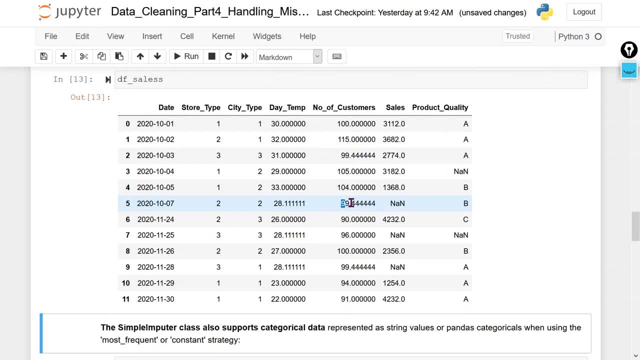 4. both column will be included here. You can see both missing value have been imputed: 99.44.. You can see Now we will impute this product quality. it means categorical variable. How we can impute this categorical column values. 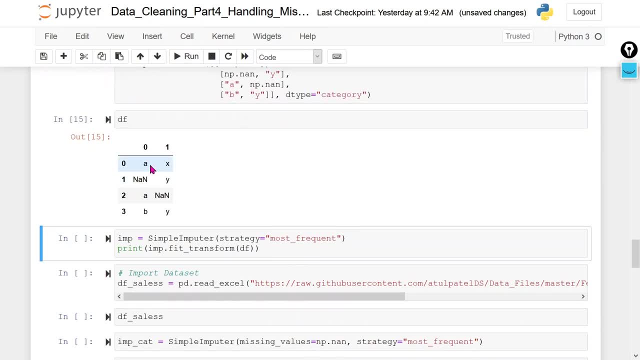 So let me first create a one data frame. You can see here there are the two column, both are the categorical. If we want to impute this NAND value or the missing value, then we will use the most frequent strategy. What it will do? 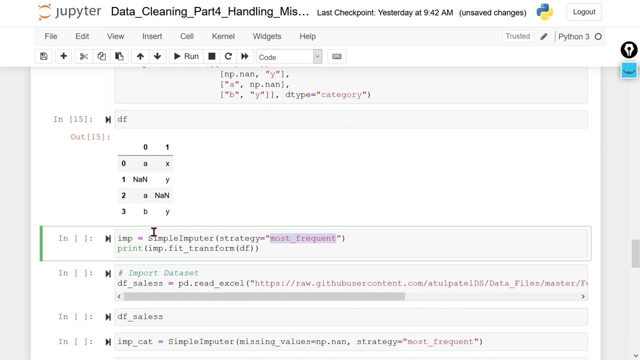 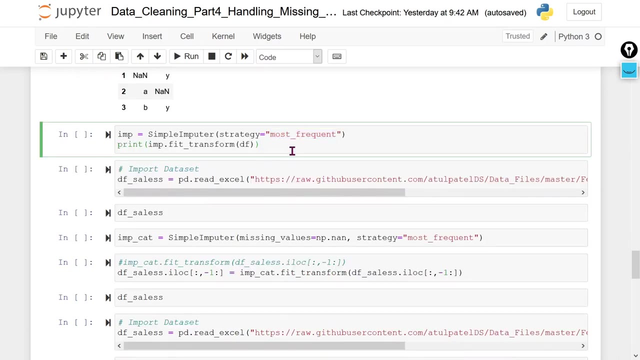 It will check what is the most frequent value In this column So we can see A is a most frequent and BY is a most frequent. So NAND value will be replaced by A and this NAND value will be replaced by BY. So let me run this. 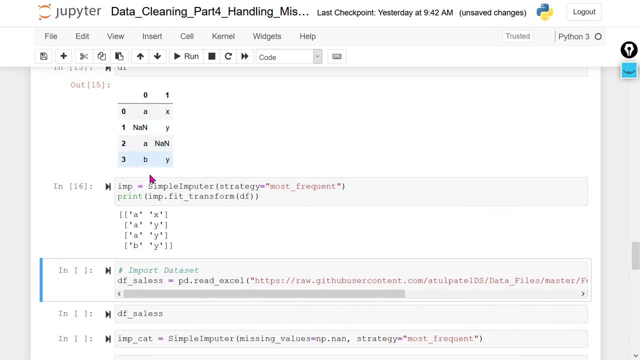 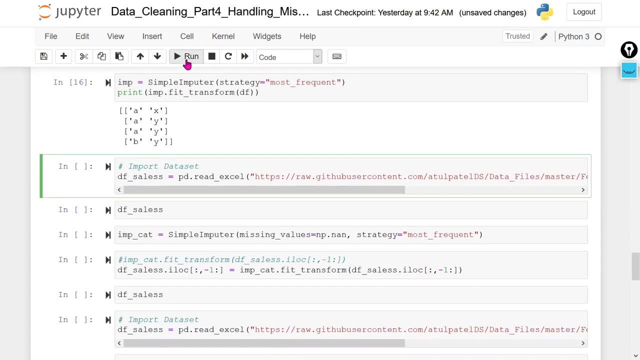 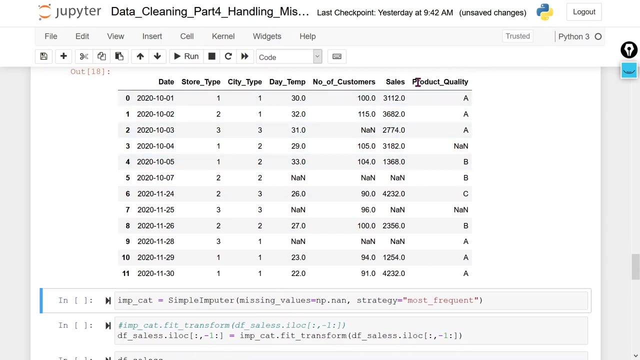 You can see A. it means this missing value has been replaced with A and this has been replaced with BY. Now I am again going to import our data set. So what I am going to do? I am going to Impute this categorical values. 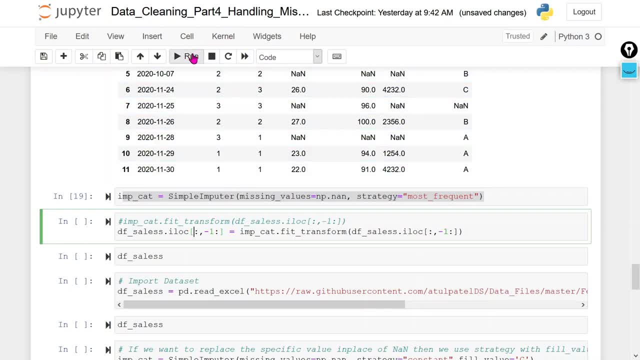 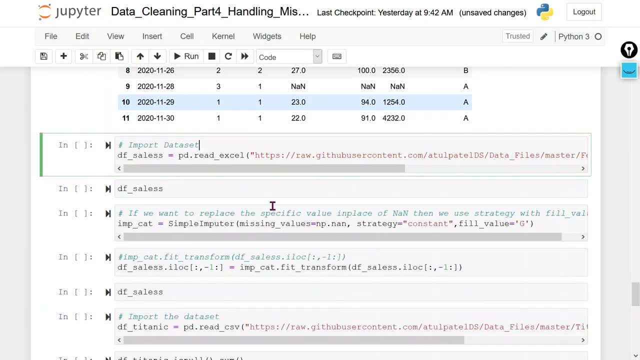 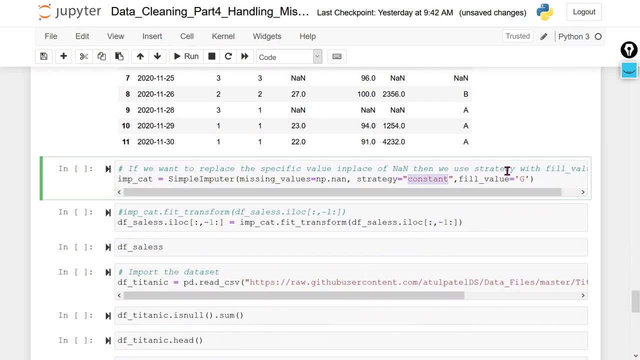 First we initialize this simple imputer, then we will fit and transform in a one go. You can see A has been replaced with missing value. Now what I am going to do, I am again going to import. Now I am going to use the constant strategy, where we will use G value to replace the missing. 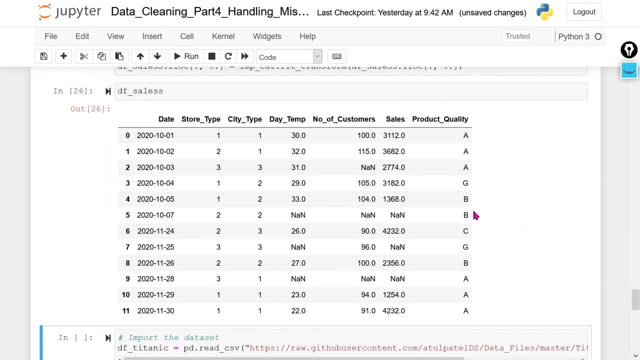 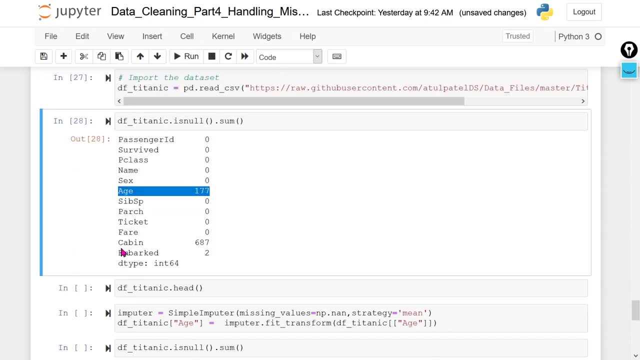 value. You can see This missing value has been replaced with G. Now again, I am going to import that Titanic data set. There are the three missing values we have. It means three column. I have a missing value, So how we can replace. 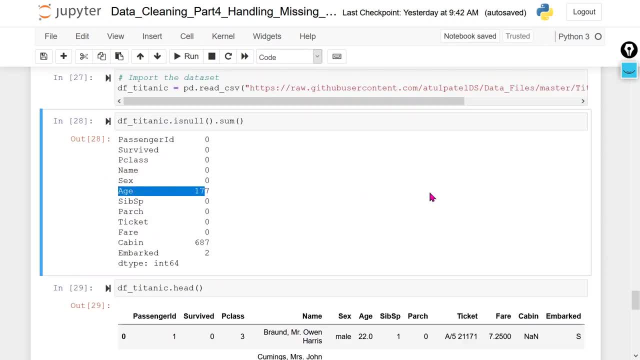 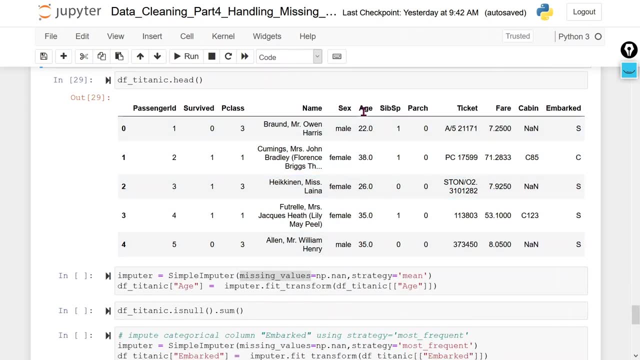 So first I am going to impute the H column missing value. So what we can do, We can take the average Or the mean of the average of this H column and whatever the value we will get, That will be Replaced with the NAND value.